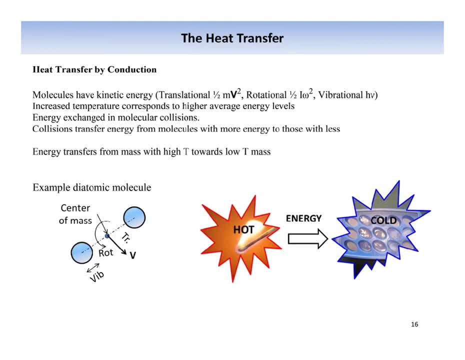 temperature difference between two systems. Heat always moves from higher temperature to lower temperature. For instance, if we have a hot copper block placed in a furnace, we initially heated it to a certain temperature using any kind of furnace. We took the block out of the furnace and placed it in a room. Now heat will transfer from, certainly the 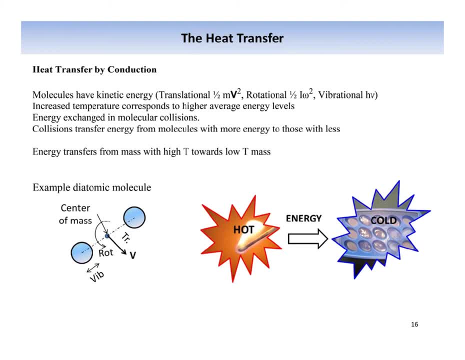 block is at higher temperature. Therefore, heat will transfer from the block to the surrounding, that is air, and whatever the surrounding is, If you place it in water, then water will be surrounding. So heat will always move from higher temperature to lower temperature. 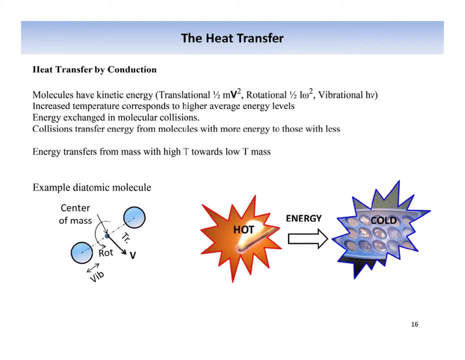 in the direction of positive gradient. Heat is transferred from the system at a higher temperature to a lower temperature, And heat occurs solely because of the temperature difference between two systems. If there is no temperature difference, then there will be no heat. There will be no transfer of heat. 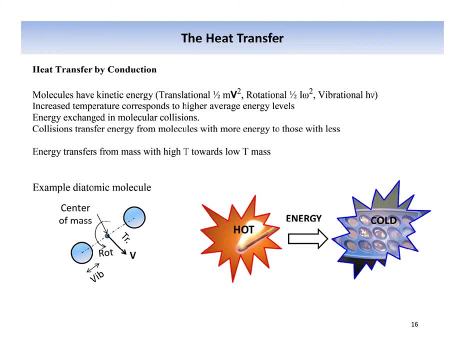 There will be no motion of heat. whatever you want to say, There will be no heat. Heat is also a transient phenomenon. It cannot be defined as a property of the system. So heat is only defined when it crosses boundaries. Another aspect of heat is that the body never 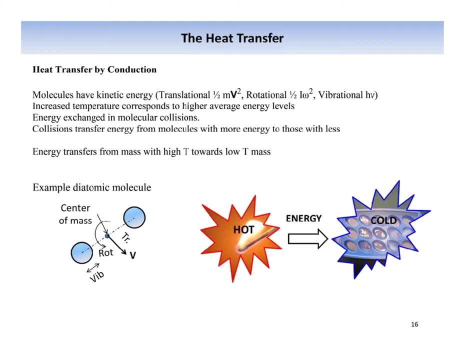 contains heat. Rather, heat can be identified only if it crosses the boundaries. Thus, heat is a transient phenomenon. If we consider the hot block of copper as an example, and the cold water in the beaker is another example, When we now put the hot copper block in the beaker filled with water, the heat will only 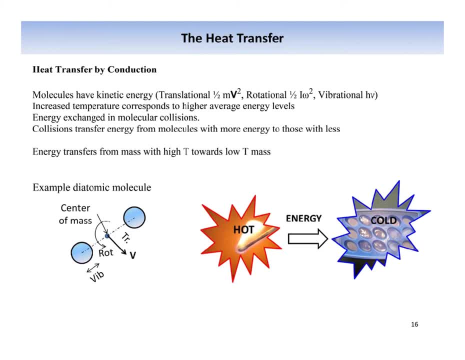 be defined when it will be transferred from copper to surrounding. Now initially assume that the copper block is at, let's suppose, 400 degree centigrade and our beaker is on room temperature, let's say 25 degree centigrade, When we initially put the block in the water. 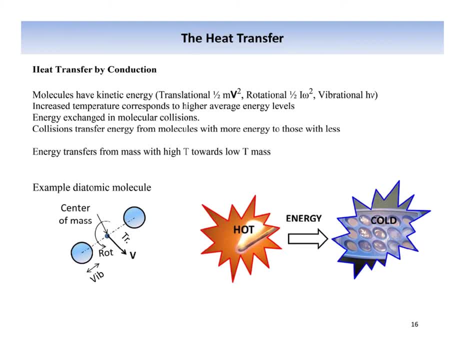 because of the temperature differences, the heat will move from copper to water, And it will continue to move until the water reaches the same temperature as of the copper block. Now the temperature of the copper block will continue to decrease and the temperature of water will continue to rise, And they will meet at a conjunction that is defined as the. 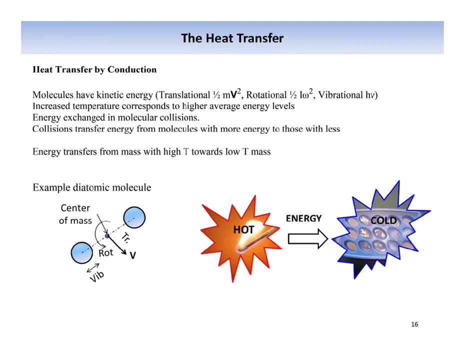 thermal equilibrium. Now, thermal equilibrium, as we have already discussed in the classes, on-campus classes, thermal equilibrium is defined when there is no temperature difference between two bodies. So we can say that the two bodies are in thermal equilibrium with each other. So heat is only defined when the copper block will have the same temperature. 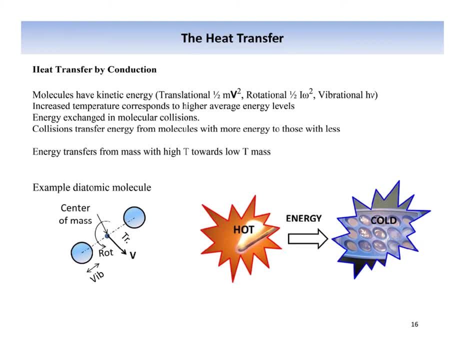 as the water in the beaker. then there will be no motion of heat. We cannot define heat at that point as a property of system. So heat cannot be defined as a property of system. So heat is a form of thermal energy. There are various forms of energy, as we already. 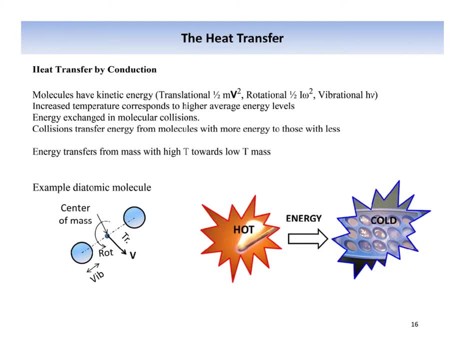 know. So heat is associated with the thermal aspect of the energies, And if we want to quantify the heat then we would require certain units. For example, in an international system, the unit of heat is joules, And the joule is defined as…. And there is another. 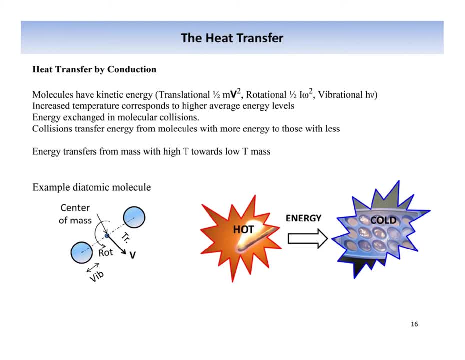 unit of heat that is known as calorie, and calorie is defined as the amount of heat required to raise the temperature of 1 gram of liquid water from 14.5 degree centigrade to 15.5 degree centigrade, by a difference of 1 degree centigrade. so 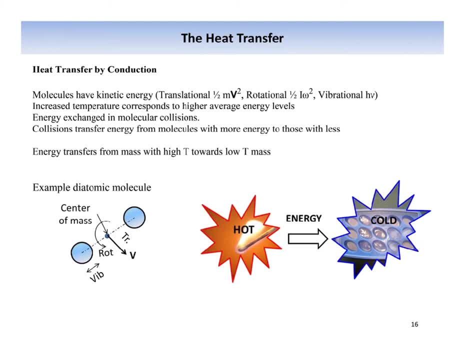 the. so we can also define that the calorie is the specific heat of water at 14.5 degree centigrade or nearly 14.5 degree centigrade. so if we wanna heat the water- liquid water- from 14.5 degree centigrade to 15.5 degree centigrade, 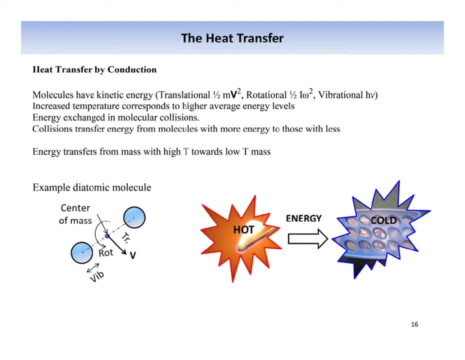 there's a one degree temperature difference. we will. so you will note that this is the same definition of specific heat, so you can also say that the calorie is specific heat at constant volume of a water- liquid water, at 14.5 degree centigrade. we have already discussed, and we will also discuss in next slides, that the 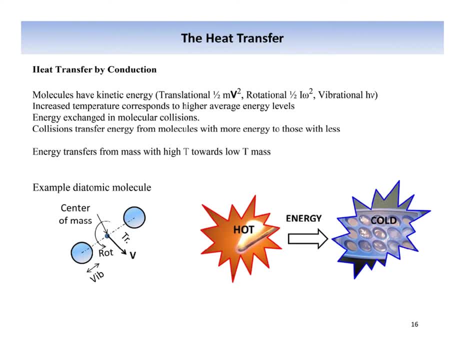 specific heat is a function of temperature. so specific heat is not constant. it varies with temperature, so we will discuss it in later slides. similarly, if you want to define the kilocalories, the kilocalories are amount of heat required to raise the temperature of 1 kilogram previously it. 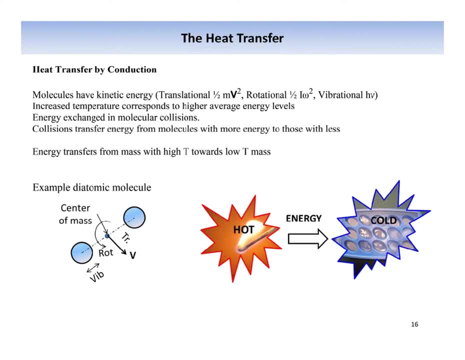 was 1 gram in the case of calories. now it is 1 kilogram of water, liquid water, to raise temperature from 14 degree centigrade to 14.5 degree centigrade to 15.5 degree centigrade. it is known as: 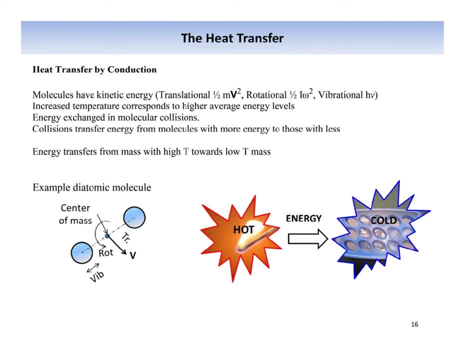 kilocalories, there's another, there's another unit of, there's another unit of heat, that is British thermal unit. it is defined as now to understand the British thermal unit heat and we will also consider the same system of hot copper block and beaker filled with water. now consider that the water is initially at 15, sorry, 59.5. 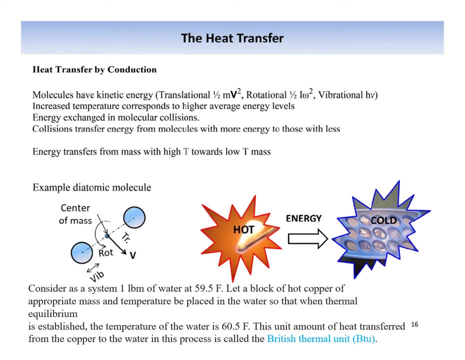 Fahrenheit and the amount of water in a beaker is one pound. when we put in the hot copper block, the rate in water temperature is 1 Fahrenheit. that is 59.5 to 60.5 Fahrenheit. now the amount of the heat that is transferred from the copper to water to raise this temperature. 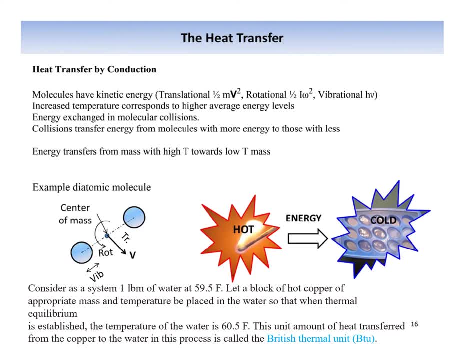 from 59.5 fahrenheit to 60.5 fahrenheit is the amount of heat. that is equal to one british thermal unit. now consider the uh. now let us talk about the modes of heat transfer. so more. there are three basic modes of heat transfer, that is, conduction, convection and radiation. for the 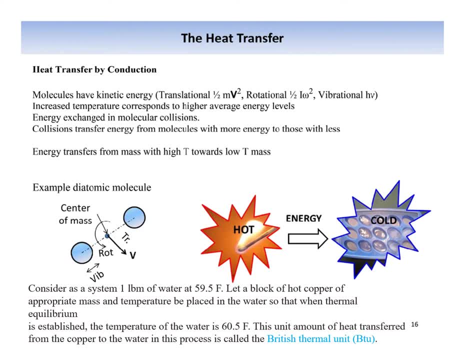 conduction case. we know that the molecules have kinetic energy, rotational energy, vibrational energy. so there are certain amount of mechanical energy that generates linear velocity, rotational velocity and vibrational motion in the molecule. so this molecule in any solid strikes the strikers neighboring molecule and transferred energy, some of its energy, to the neighboring molecule. this form of energy that 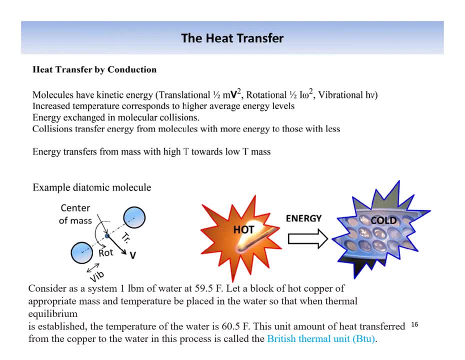 is being transferred from molecule to other molecule, while both the molecules maintains their initial position, they only strike each other, they strike neighboring molecules. this form of energy transfer is recognized by conduction as the conduction heat transfer mode. so if we want to consider an example, let us consider an example of a solid aluminum rod. 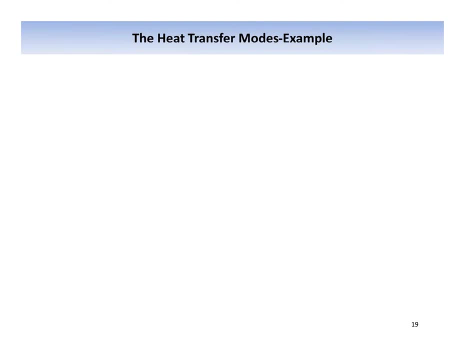 this rod, solid aluminum rod is- is placed uh on a fire of certain flame- uh, let's uh the natural gas flame and uh let's suppose the uh this, uh, this end of the rod uh is uh at 400 degree centigrade and the other end of the rod is placed in. 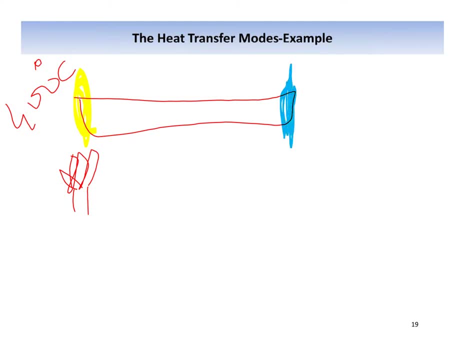 theимсяiss mimetic in an ice bath having temperature of zero degree centigrade. so heat will transfer from 400 degree centigrade to zero degree centigrade and the molecules if we, if we take, and here this, which is a magnifier, 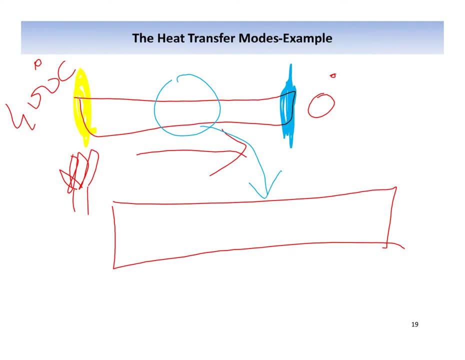 large of 125, magnitude, 500, bonaمة of 300 would have had done this. 15ら considers, we consider these molecules and again we consider these two molecules, and rotating and vibrating at a frequency and banging its neighboring molecules and transferring energy in this form. this is conduction heat. 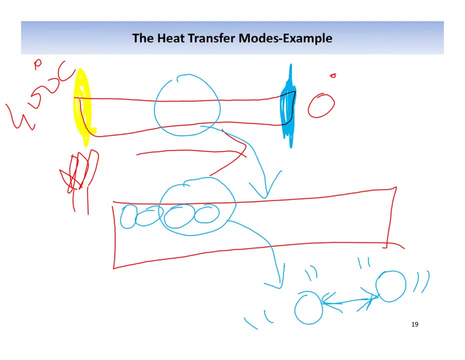 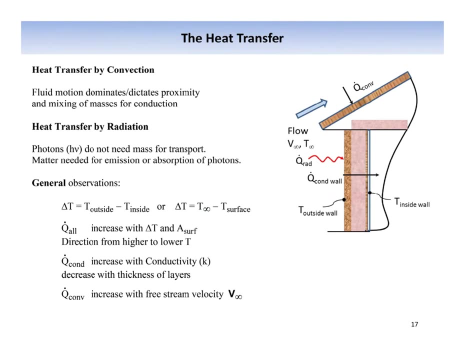 transfer mode. it is recognized a mode of conduct, a mode of heat transfer name conduction. a second heat transfer mode is convection, and in convection the molecule physically moves from one position to another and carries energy with it, and this form of heat transfer is known. 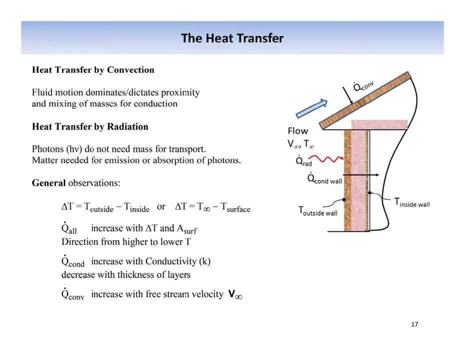 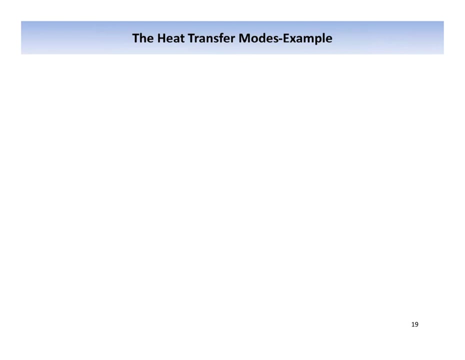 as convection, for example. for example, we considered a hot copper block example when defining the units of heat and we we put a hot copper block in a beaker filled with water. now, the now, if we consider, if we consider the hot copper block being placed in and this beaker filled with water, and here hot copper. 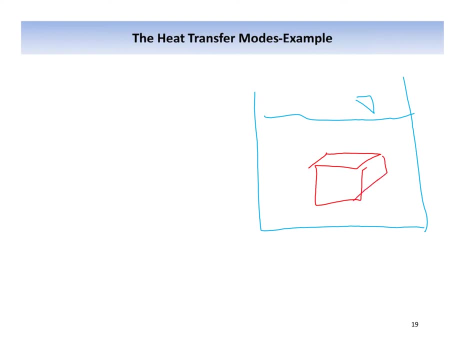 block is placed. and if we magnify this wall and talk about water molecules- here hot copper block is placed and if we magnify this wall and talk about water molecules, so this molecule will physically move, it will take energy from the wall and it physically moves upward. this molecule will be replaced by another molecule and 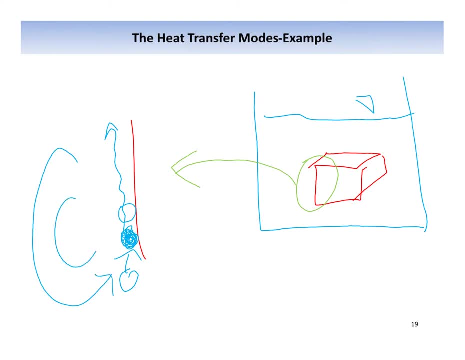 this will convert. this will generate a motion in the medium in which the molecules changes. molecules change their initial position. this mode of heat transfer is known as convection, where the medium facilitates a transfer by its motion. and there are two form of heat convection. one is free convection or natural convection, and the second one. 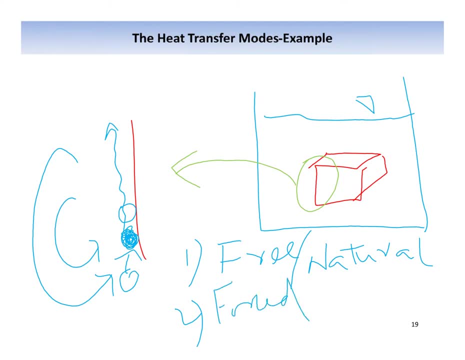 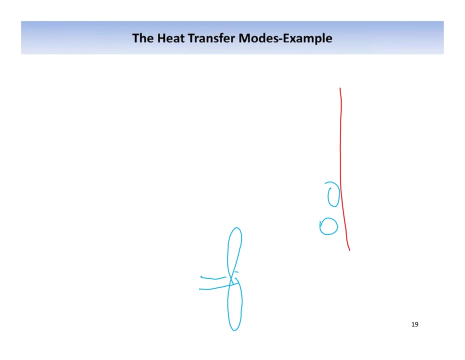 is forced convection. now let us define what is free convection and what is natural convection. free convection is the. what is what we have considered? this example that we have solid glass and hahahaha. for example, that 하기 vora forces the molecule to strike this wall and take energy and and complete this phenomenon. now we 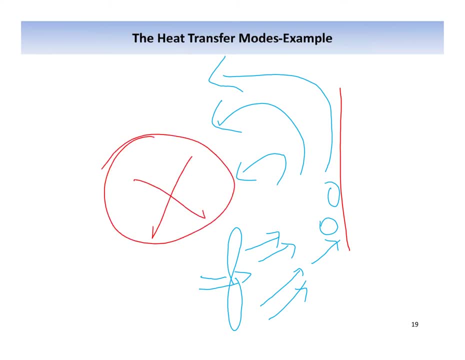 we didn't. we didn't use a propeller or any sort of any sort of source that generates the motion of medium. so this is, if you don't use- and it's any- any source and we do not force the medium to move, it moves by itself. it moves because because when this molecules takes energy from the wall, 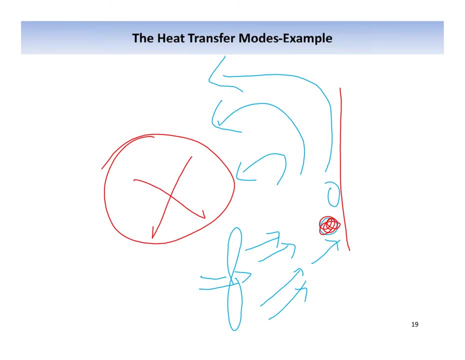 and there will be a local difference of densities there, uh, of a hot medium and a relatively cold medium over here. let's suppose so, because this medium, this portion of medium, will have higher density, so the molecule will will move down because of higher density and this low density molecules will move upward. this is called nasal convection. 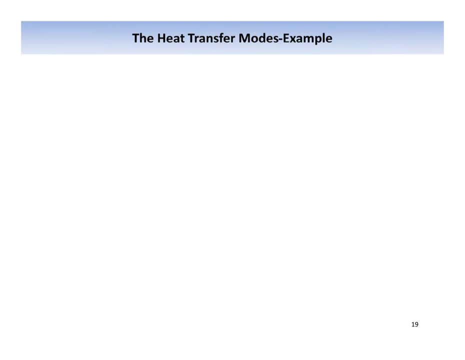 on the other hand, if we consider force convection, for example, we have, we have a heat exchanger and we have this shell and tube heat exchangers in which we have these different tubes, this shell and tube heat exchangers. we have these tubes and let's suppose water at 40 degree centigrade. 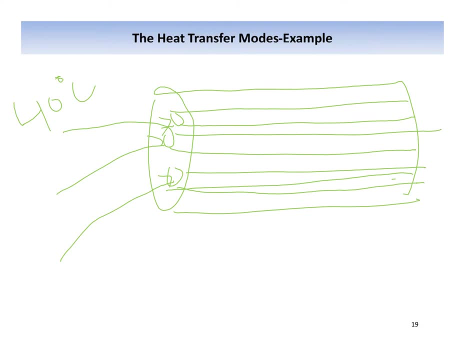 enter it and we use, enter these small tubes in this big tube. there is water at zero degree centigrade, there is water in 0 degree centigrade and what we are doing? what we are doing is we are we are forcing this water to enter, this cold water, to enter from here and leave this so in the. if we look into the cross sectional view, 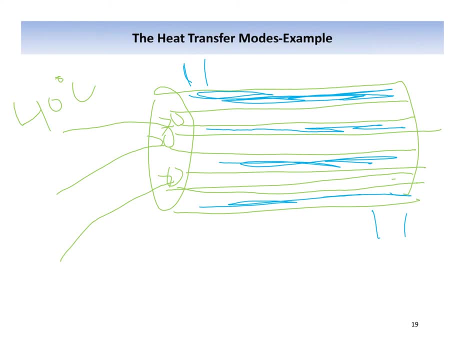 that was the water that was about to send. right now we have to put it into the water tank. So if we look into the cross-sectional view, this big tube and there are small tubes in it. In these small tubes there is water flowing at 40°C and another liquid, that is water, at 0°C or 10°C. 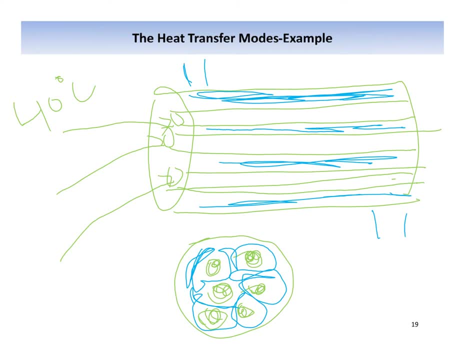 That is a relatively small liquid. So if we look into the cross-sectional view, this big tube and there are small tubes in it, Groovy and warm And the cooler then 40°C is moving. in this shell There are small tubes and then there's a big shell. 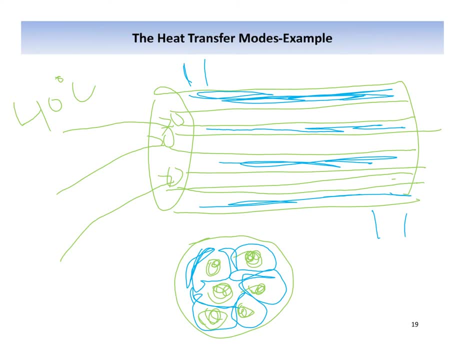 water at 10°C is cold water in the shell and water at higher temperature- 40°C- is water in the tubes. a pump: we are using a pump to to pump this cold water and obviously, this hot water as well. now we are forcing the molecules of cold water, molecules of 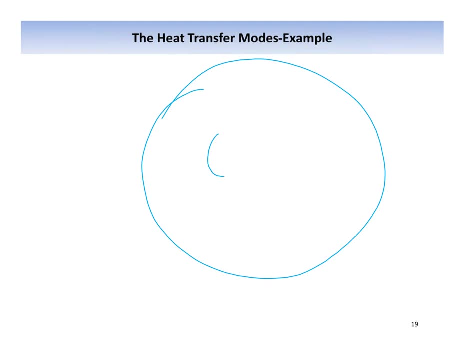 cold water to strike these tubes, wall of these tubes, using pump. so we are using and move on and move on. a new molecule will replace it. but we are forcing this new molecule, we are generating this motion of water to expedite, to facilitate, to enhance the heat transfer. so this type of heat transfer is known. 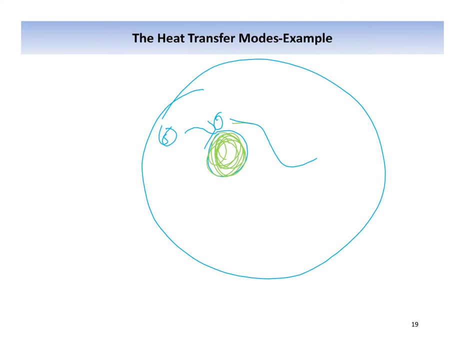 of heat transfer, or this type of convection is known as forced convection. now there is another form of heat transfer, that is heat transfer because of radiation and radiation heat transfer. in radiation heat transfer we do not require any medium, for example in convection and in conduction. we 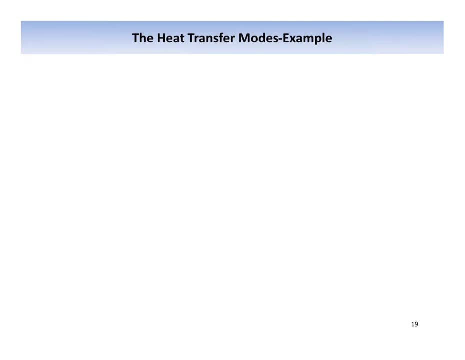 discussed examples that the heat is being transferred from higher temperatures to lower temperatures using aluminium solid rod. solid rod is a medium, and then we in convection we considered an example in which we placed a hot copper block in a cold water medium, and the These types of heat transfer require certain medium to transfer the heat from higher potential to lower potential. 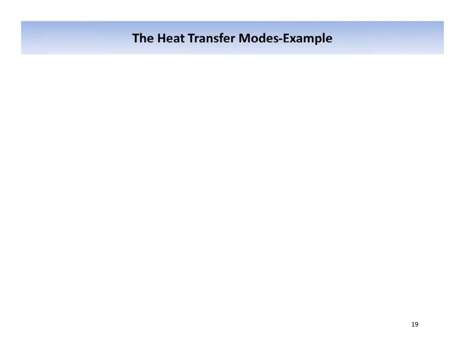 However, in radiation, we do not require any source of medium, any sort of medium. For example, let us draw a globe. This is Earth, If we can draw it as we can. This is Sun. Radiation is the main medium. This is the main cause that we are getting energy from Sun to the Earth. 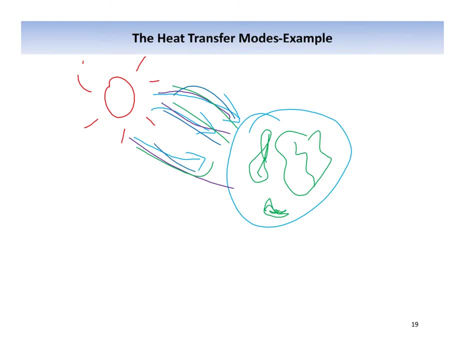 While there is no medium in between Sun and Earth, Heat is being transferred from high temperature, that is, Sun, to low temperature of Earth, But there is no medium in between. So this type of heat transfer is called radiation heat transfer. It only depends upon the temperature difference. 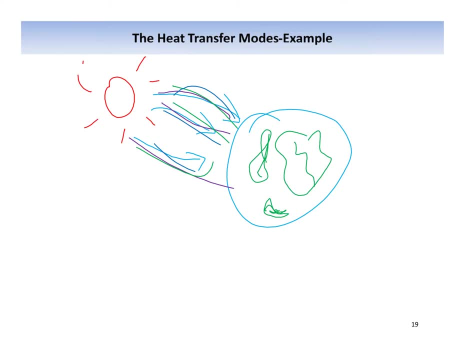 For instance, we have a radiation source over here And then, And then, And then Its temperature is 400 degree centigrade. And then we have some body over here that has a temperature of 10 degree centigrade. Now the radiation will. 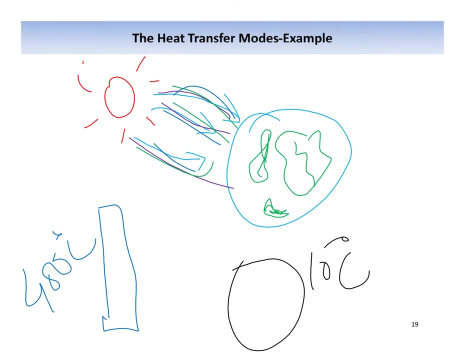 And there is no medium in between. The amount of heat transfer that will transfer from this high temperature to low temperature using radiation only depends upon the temperature difference. This 400 degree centigrade and 10 degree centigrade. There is a temperature difference of 390 degree centigrade. 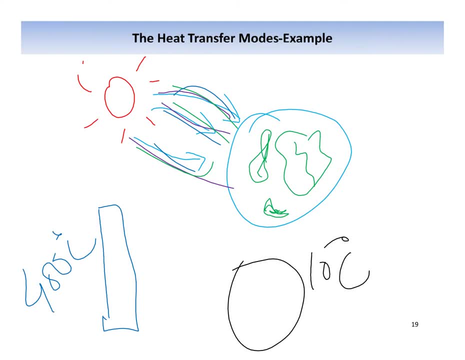 It exactly not depends upon the temperature difference. It depends upon the temperature difference After taking its power to the 4.. Now we will discuss it in the next coming slide. So what is the temperature of higher body? What is the temperature of lower body? 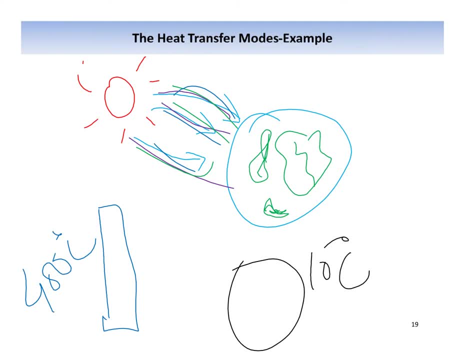 The greater the temperature difference, the greater will be the heat transfer because of the radiation. It also depends upon emissivity. What is emissivity? Let us discuss shortly. And then there is the frontal area. What is the exposure area between these two bodies? 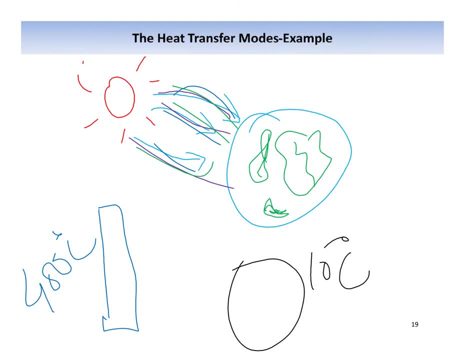 If there is a certain hindrance in between, For example there is a wall in between, Then there will be substantially low amount of heat transfer. So, depending upon the material of this wall, Either it allows the radiation to pass or not. 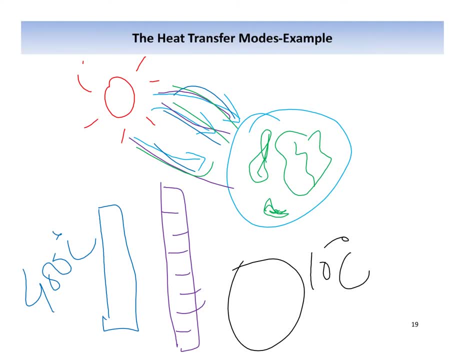 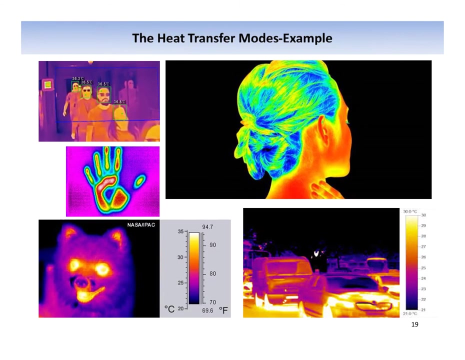 If there is less exposure area, Lesser the exposure area, lesser will be the heat transfer because of the radiation. So what is emissivity? Now, in this slide we can see different images that are being generated by thermal imaging camera And it senses the radiation that comes out of the body. 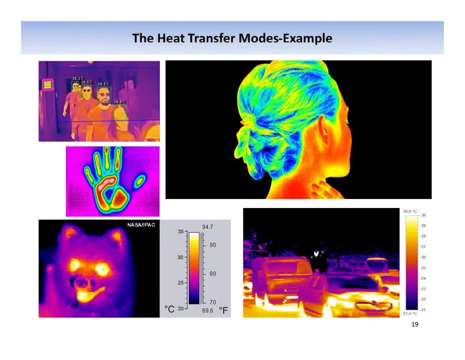 So we can see that there are different pictures: A picture of a lady, Some guys coming out of a gallery, A dog, a hand and automobile vehicles at road. We can see that How the thermal imaging camera senses and generates these images. 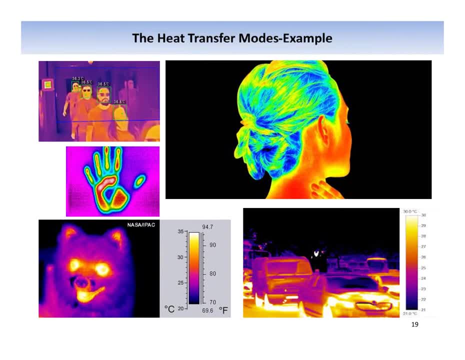 It takes the radiation coming out of the body And it puts that radiation in a perspective And do the math. Let us see these pictures. We can measure temperatures Using these non-contact type sensing techniques. We can see that the engines are heated. 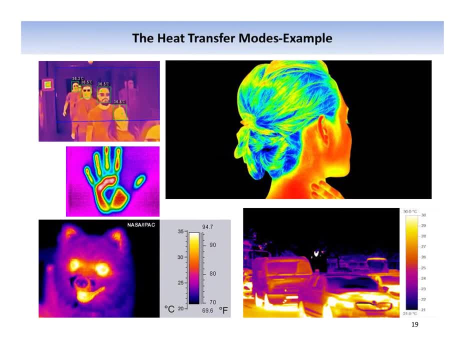 Because of the temperature. Then the front portion of the car is bright yellow And there is less amount of thermal energy in the cabin, So it is like purple or black. So we can see the human hand is also generating certain radiation. 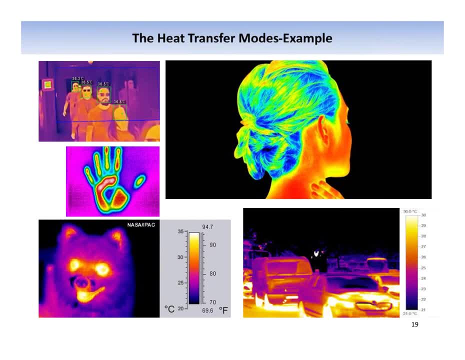 Humans are generating, Animals are generating. So every material, either engineering or non-engineering, It generates the heat, It generates the radiation. Sometimes it falls in a human visible area Or visible capability To view the color, Sometimes it is not. 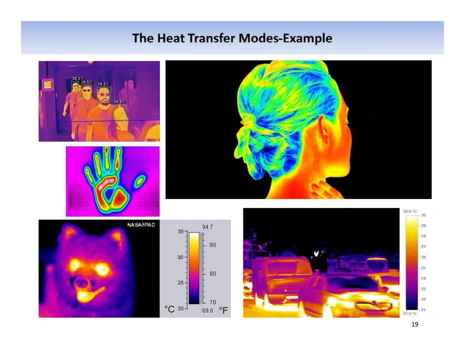 But the material generating the radiation. This is the emissivity. So the emissivity is the capability of the temperature Of our body to emit the radiation At certain temperature. Higher the emissivity, Higher the radiation heat transfer. Lower the emissivity. 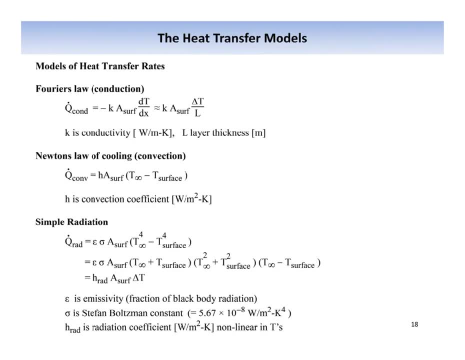 Lower the heat transfer Because of radiation. Now the formulas For heat transfer Because of conduction, convection and radiation Are presented over this slide And you can see And we will. We will discuss The What is K. 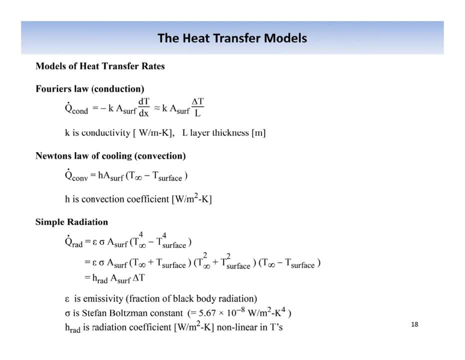 K is the conductive heat transfer coefficient. Higher the conductivity of material, Higher the value of K. A is the cross-sectional area From which the heat flux passes D and T DT over. DX Is the temperature gradient. What is the? 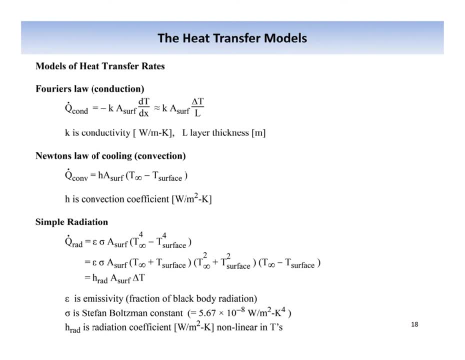 Temperature difference of two bodies And what is the distance between them And the convection H is the convection heat transfer coefficient? It depends upon Not many things And you will Calculate Heat transfer coefficient Because of You will discuss. 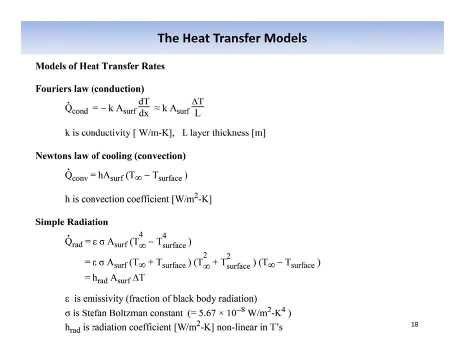 You will learn Convection heat transfer coefficient In detail In another course. That is, Heat and mass transfer. Then is A: What is the area Where molecules are being forced Or naturally Heating the surface And taking the energy from it? 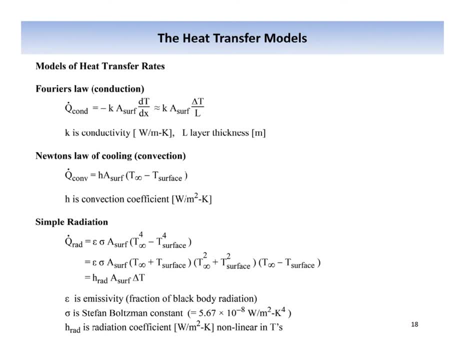 And moving on In convection, We know that The medium moves In the heat convection. So what is the area? For example, The, The. A particular example We considered In convection Was the Block of 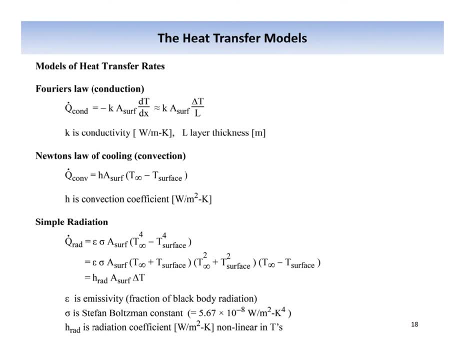 Hot copper Placed In a beaker filled With water And water is taking Water. molecules are taking Heat, So the walls Of Block- Hot copper block- Is the area From where The molecules are taking. 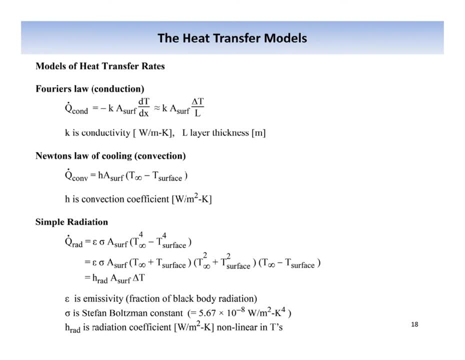 The energy. So is That area? T is T infinity. What is T infinity? T is infinity That, If We Have This, This Copper Block Wall, And Obviously It is At 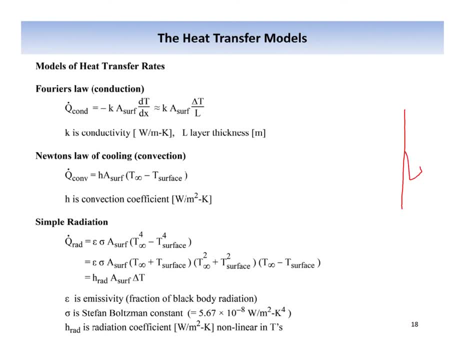 Four, It was On 400. Degree centigrade, As We Discussed. Now Molecules Near To It Will Have More Than The Molecules Relatively Away. 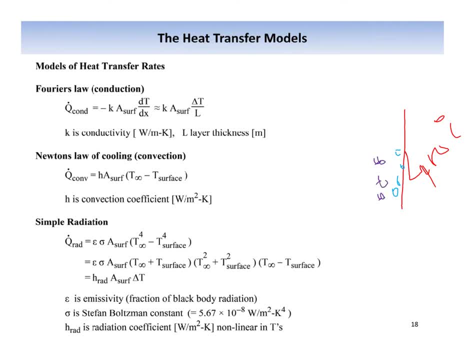 From The Wall Than The Molecules From Far Away Than The Molecules Far, Far Away. So There Will Be Temperature Difference Between These Molecule. 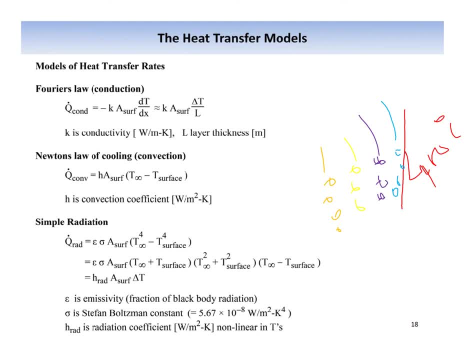 Layer, There Will Be Temperature Difference, Special Temperature Difference, Depending Upon The Special Space Coordinates. So If We, If You, Keep Moving Away From The Body, 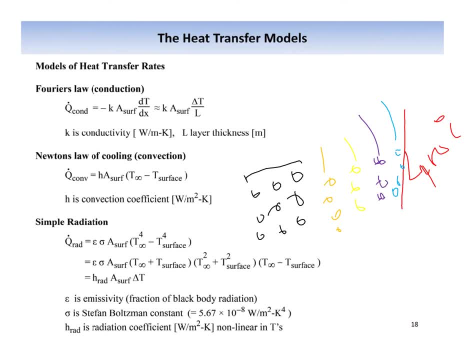 Than We Will Come From This Layer Of Molecules In Our Water Medium, As We Have Considered In This Example. So What Is The Temperature? 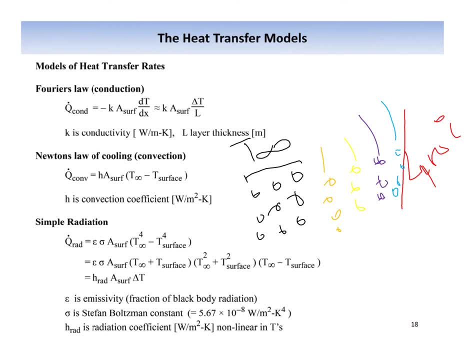 We Take As The Infinity For Example. If We Keep Moving Toward The Copper Block, We Will Observe That The Air Will Keep Getting Hotter.